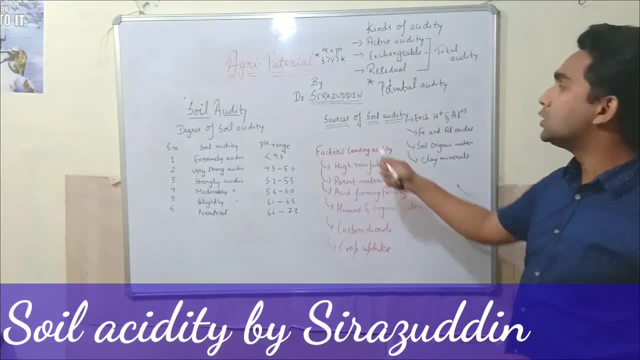 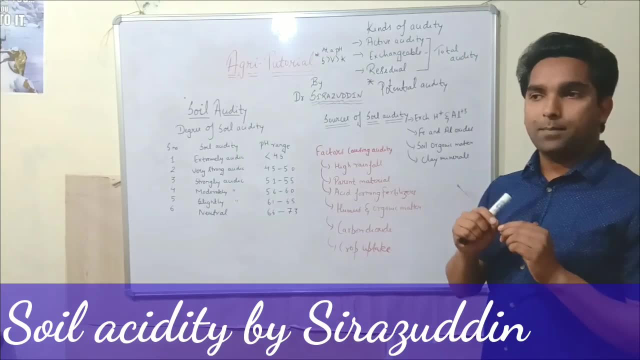 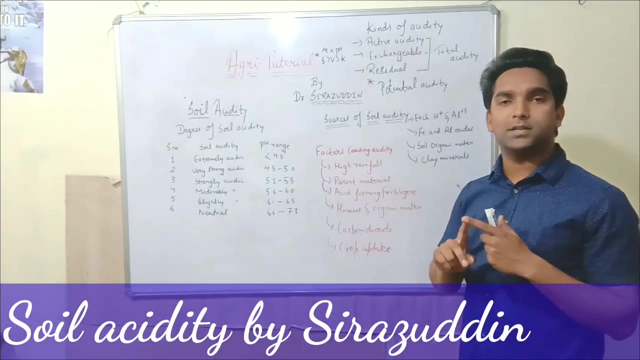 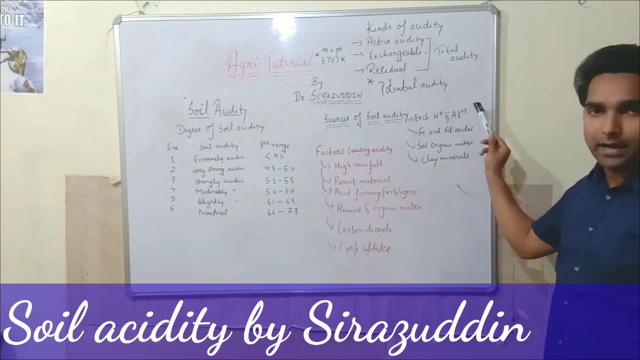 So, moving on, now we have to talk about the sources of soil acidity. Now you know that soil acidity, as I told you earlier, if your pH is less than 7, then your acidity is caused. So, basically, if we talk about hydrogen ion concentration, then the first sources are exchangeable hydrogen ions and aluminium ions. 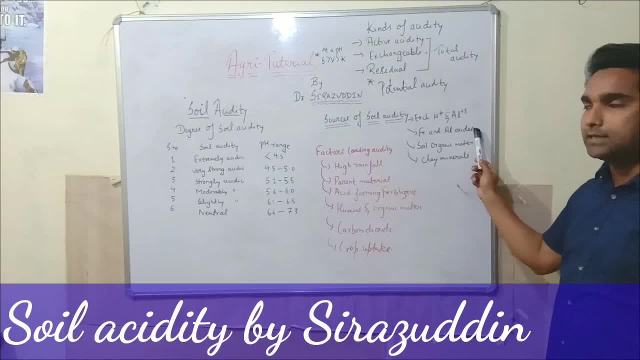 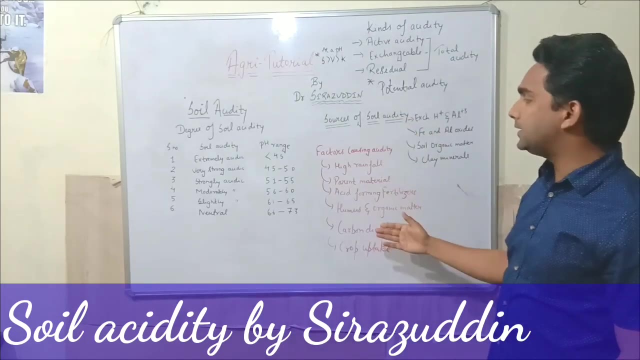 The second one is iron and aluminium oxides. The third one is soil organic matter and the clay minerals. So these are the sources of the soil acidity. So let us talk about the factors which cause acidity. So to highlight them. you see the topics. 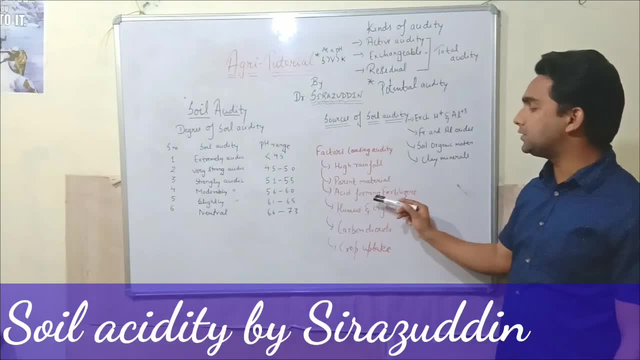 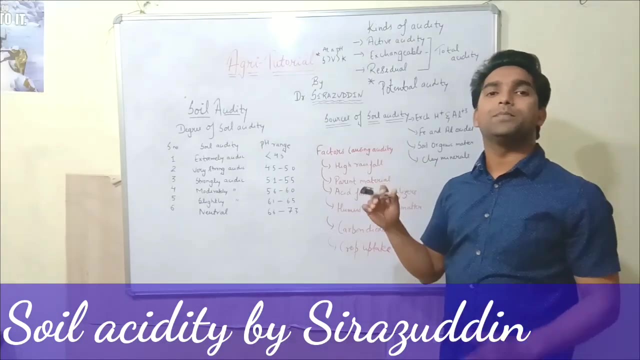 We have high rainfall, parent material, then we have acid forming fertilizers, humus and organic matter. We have carbon dioxide and crop uptake. So let us take one by one, If we talk about high rainfall, what happens, dear, when you have high rainfall, then the bases in your soil will lose down. 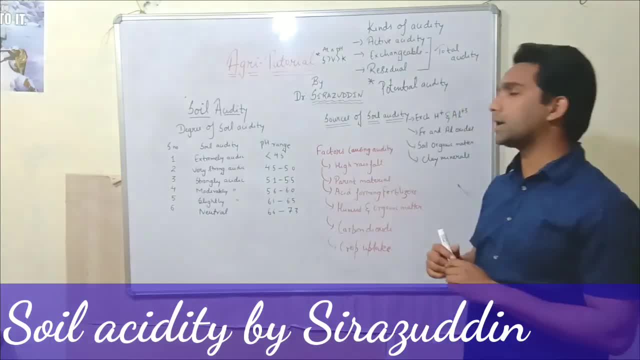 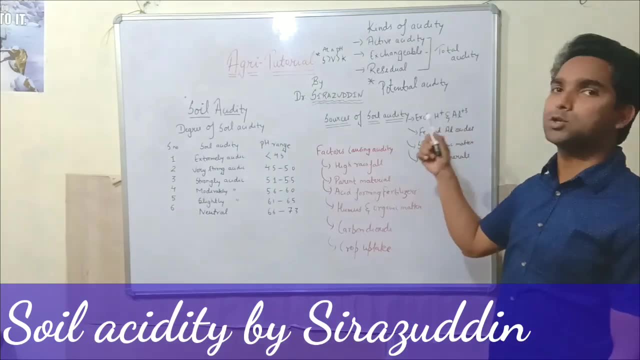 And when they go below the root zone, then what will happen? Due to the lack of exchangeable bases, the concentration of hydrogen and aluminium oxides, or ions, will increase in the soil and that will cause, or that will add to the acidity of the soil. 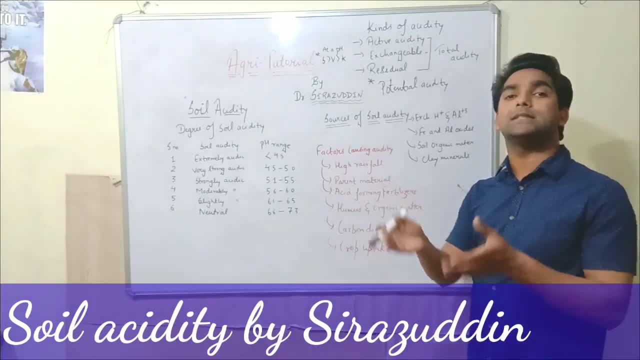 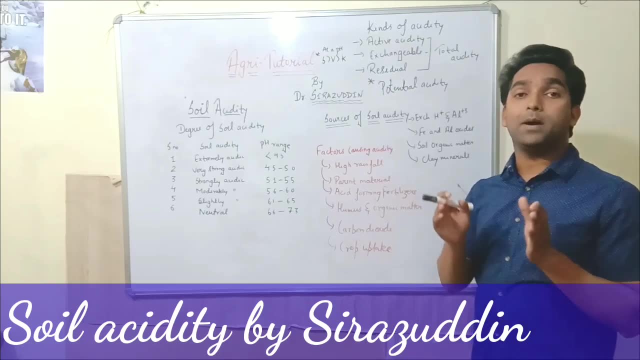 Then parent material. If the parent material is acidic in nature, then certainly the soil is also acidic in nature And, for an example, if your parent material is made of graphite, then whatever soil is developed from those logs, that will also be acidic. 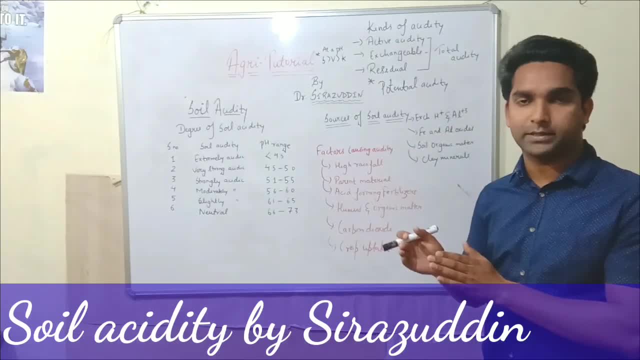 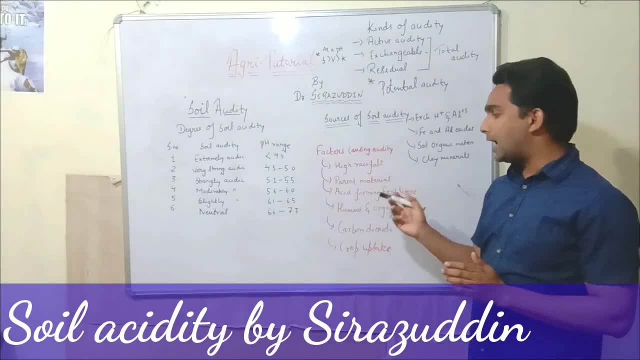 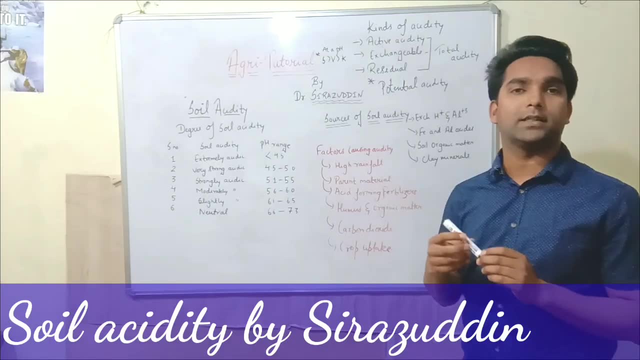 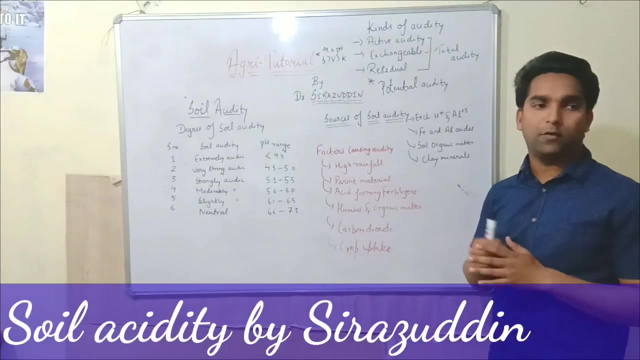 Then acid forming fertilizers. So you can say this also related with anthropogenic activities. If you use some of these fertilizers in the soil, which generally causes acidity, then you will increase the acidity. So basically, if the fertilizers of the ammonium forms, they cause acidity. 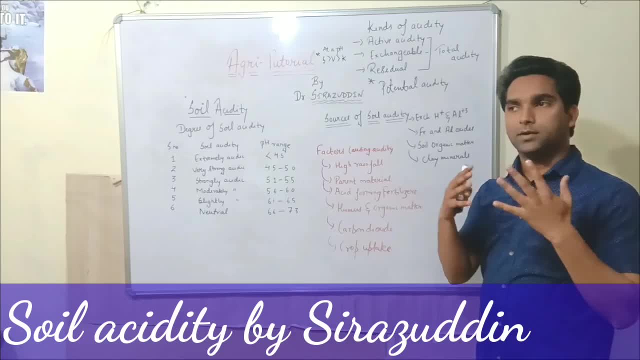 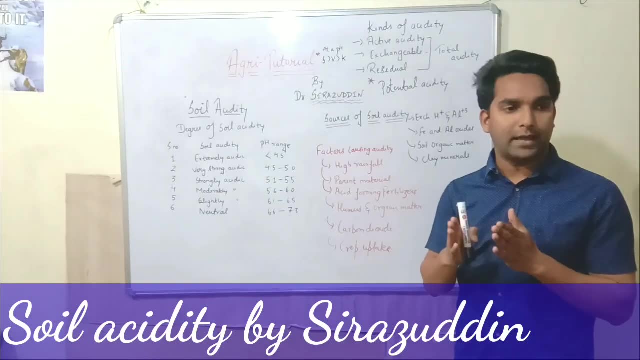 So ammonium sulphate, ammonium nitrate. they generally cause acidity And you might be thinking: why are these so acidic? and you might be thinking: why does this happen? so whenever you see that your ammonium ion is a cation, so when you add cations, 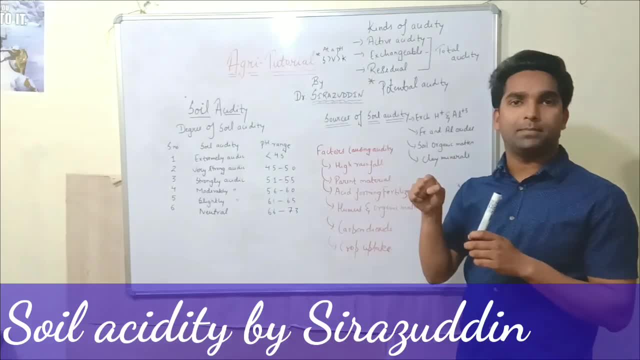 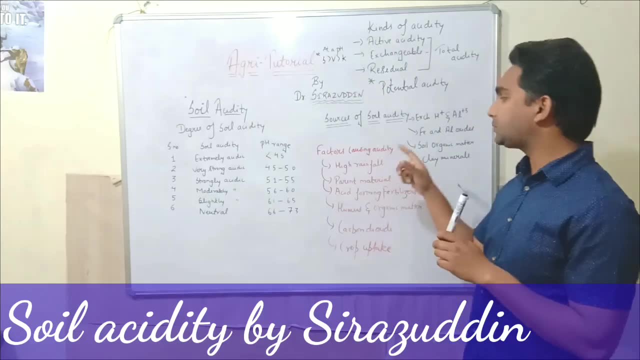 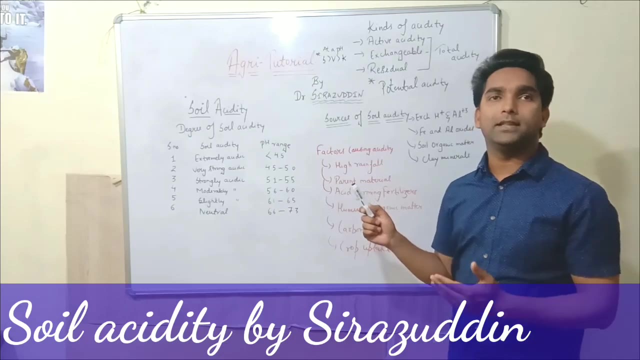 so in compensation. when the plant is taking cation, so in compensation to balance it, hydrogen ion will release in the soil and that will cause the acidity. so it means we should use nitrate fertilizers in acidic condition rather than the ammonium form, then humus and organic matter. 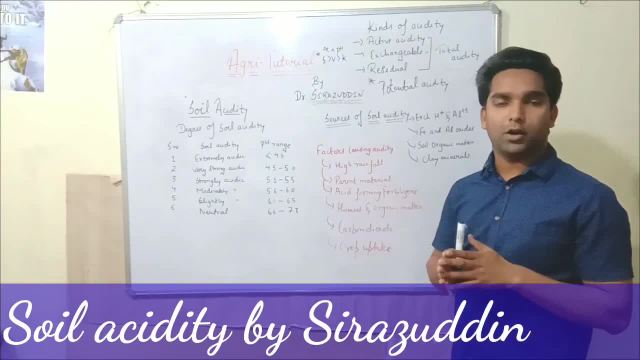 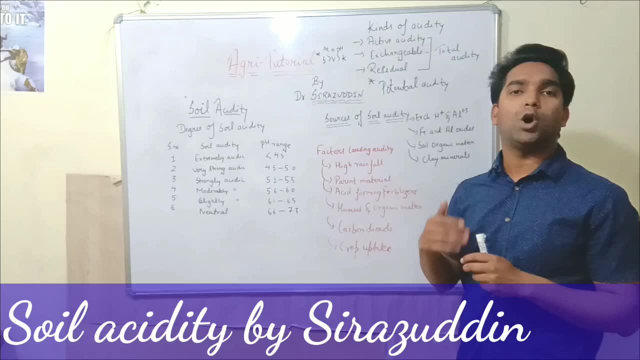 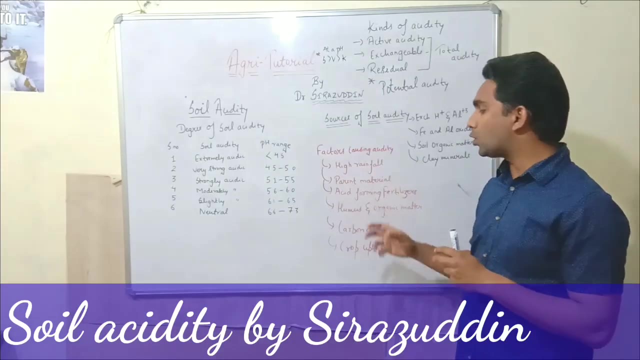 we know that humus is the final product of the decomposition of the organic matter. so what happens is that when the organic matter decomposes, it releases some organic acids. if it releases organic acids, then that will add to the soil acidity. moreover, the humus and organic matter 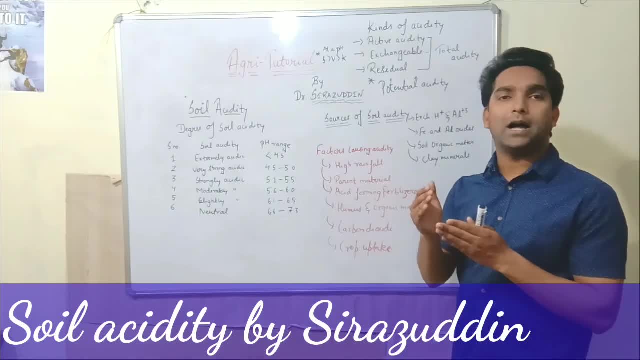 when it decomposes. so it has got carboxylic group, it has got phenolic group and it also has got enolic group. these three groups, these are the functional groups. they can attract or dissociate the hydrogen ions, so that will also cause the soil acidity. 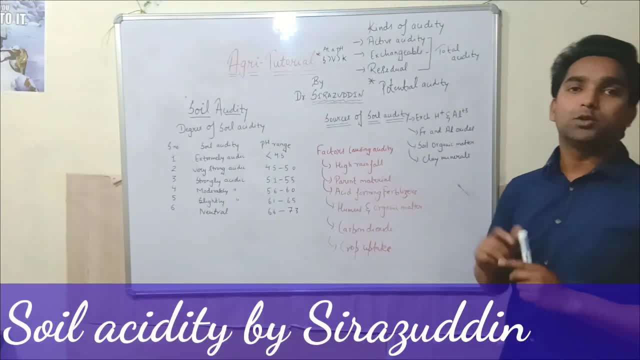 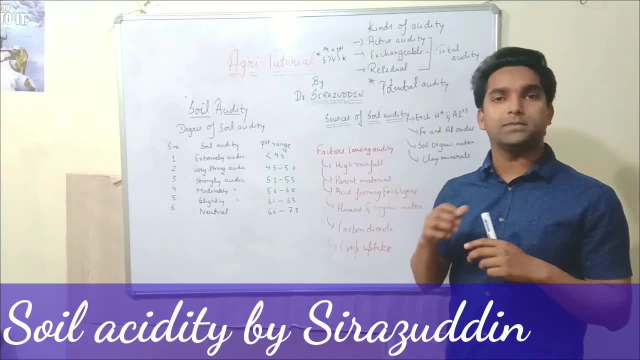 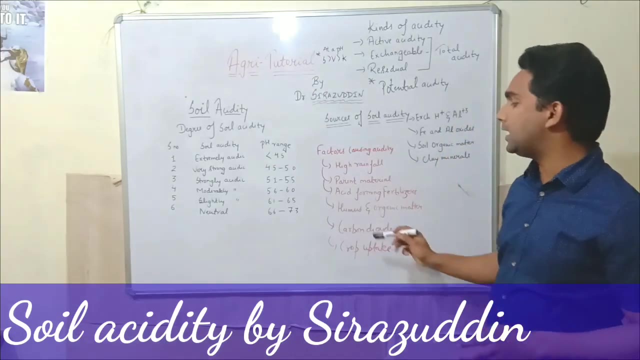 moving on, we know that carbon dioxide. so now you might be thinking: where will the carbon dioxide come from? so you know that the soil respires and, moreover, your microorganisms respire, your plant roots also respire, so from their respiration CO2 will come that will react with the water. 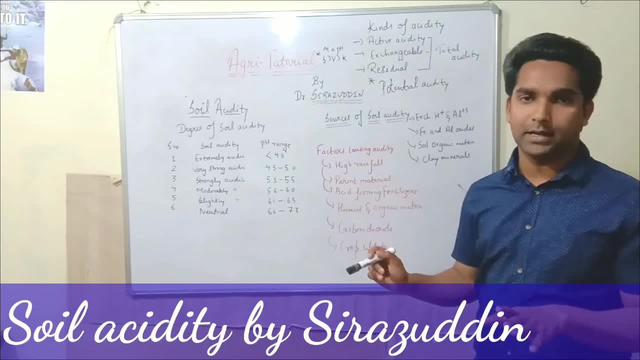 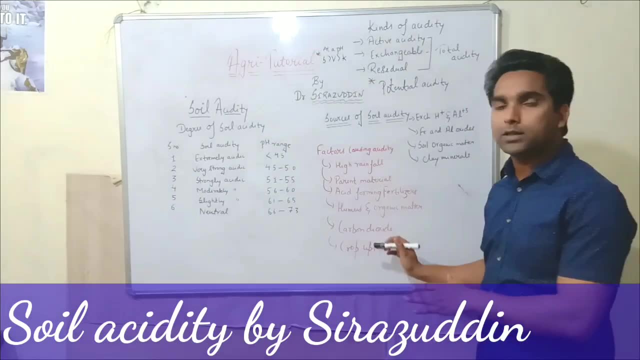 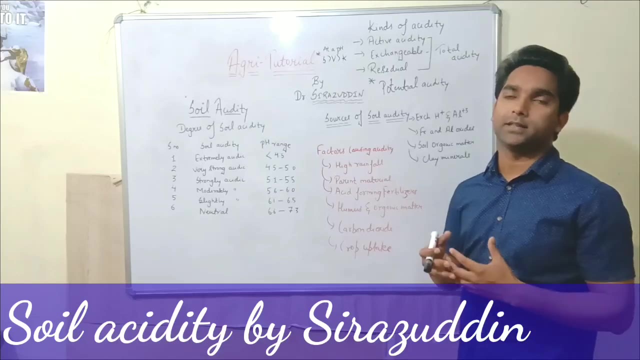 and that will form H2CO3, that is the carbonic acid. so carbonic acid also causes the soil acidity. and the last one is crop uptake, and this is a very important point because some crops are such that prefer to uptake the divalent cations. 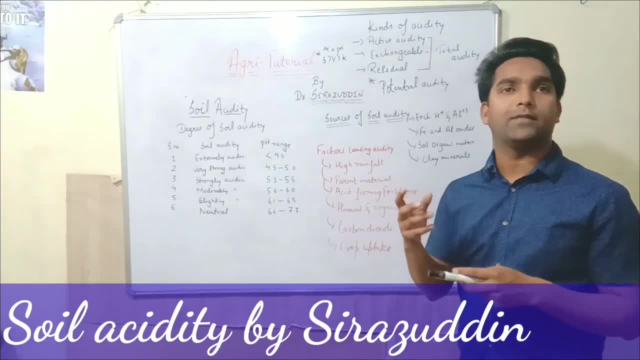 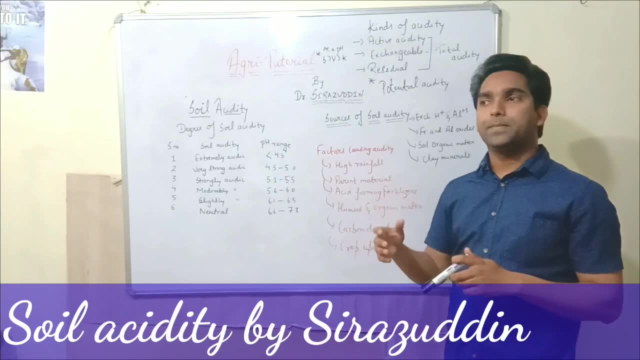 so, in case of divalent cations, we have calcium, we have magnesium and these are bases. if any crop uptakes these, then your bases will ultimately lack in the soil and will cause acidity. moreover, most of the legumes they have got higher CEC, their root CEC. 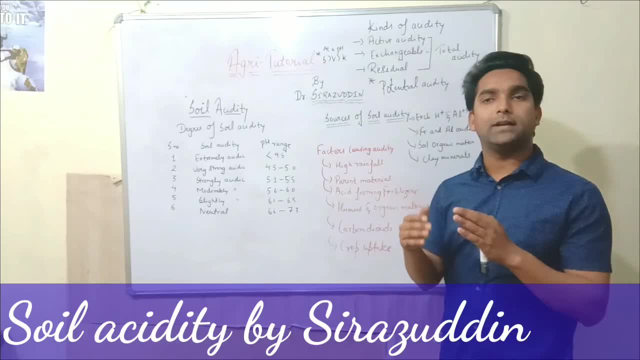 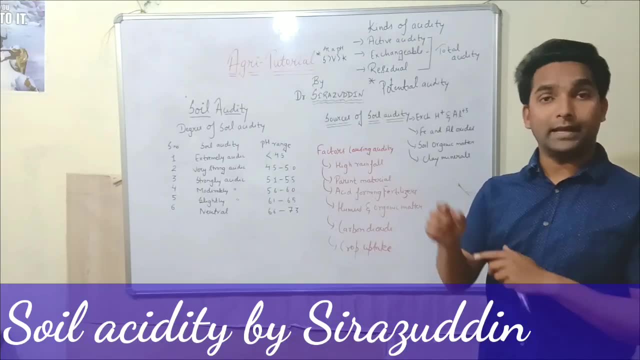 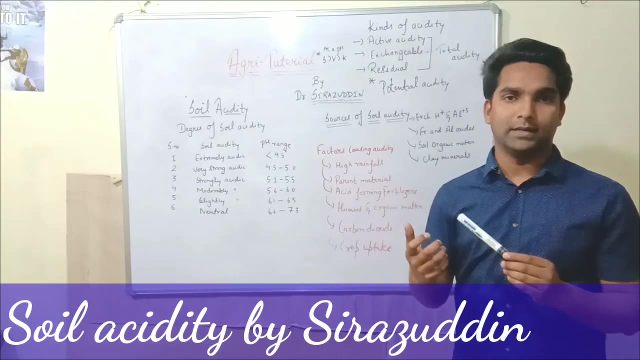 is higher in comparison to the cereals and that is why they prefer, you know, a divalent cation uptake more rather than the monovalent cation. but in the case of cereals it is the opposite: your monovalent cations uptake is more in cereals. 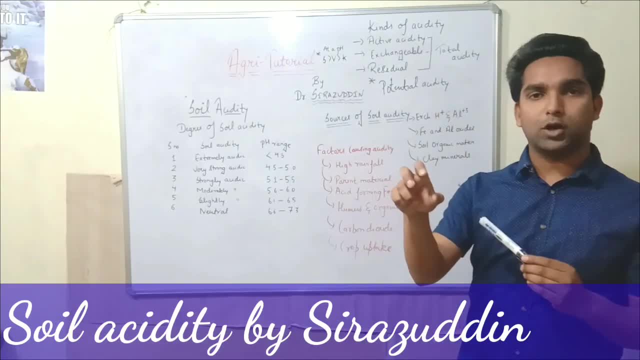 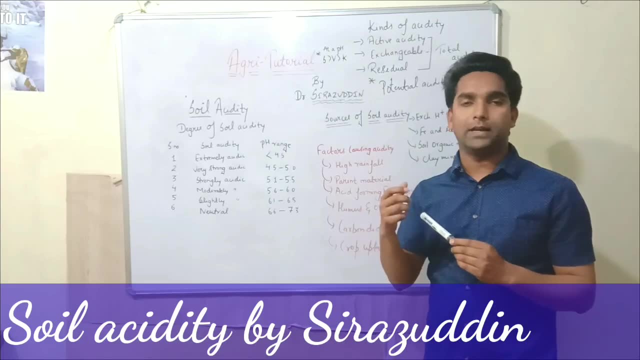 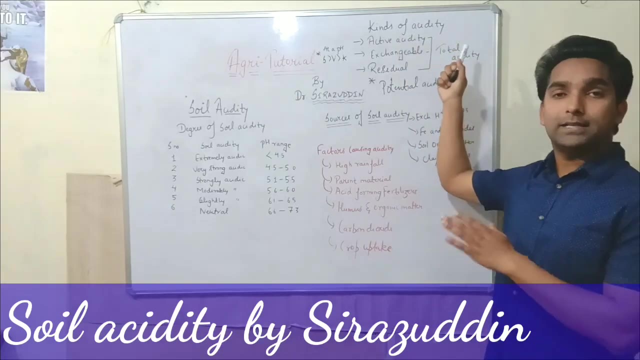 so you have to remember: leguminousy crops: they prefer uptake of divalent cations. cereal crops: they prefer the uptake of monovalent cations. now, after this, we will be dealing with the kinds of acidity and the soil science group who are preparing for agronomy. 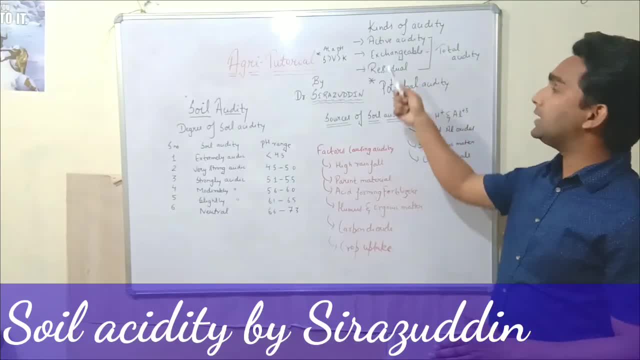 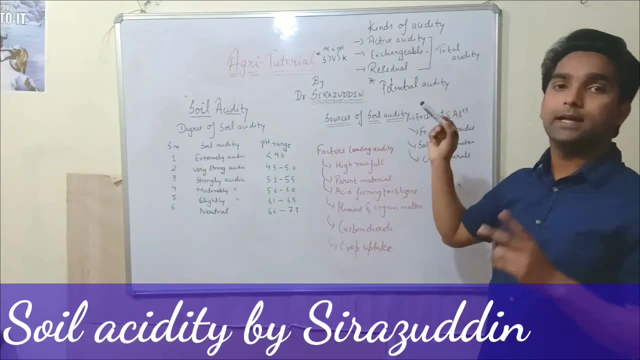 with SRF generally, one or two questions are frequently asked. so let us start that there are basically three forms of acidity. first one is active acidity, another one is exchangeable acidity and the third one is residual acidity. so let us take them one by one. now we will talk about active acidity. 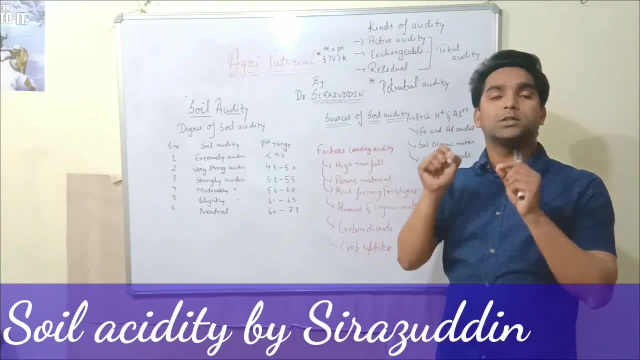 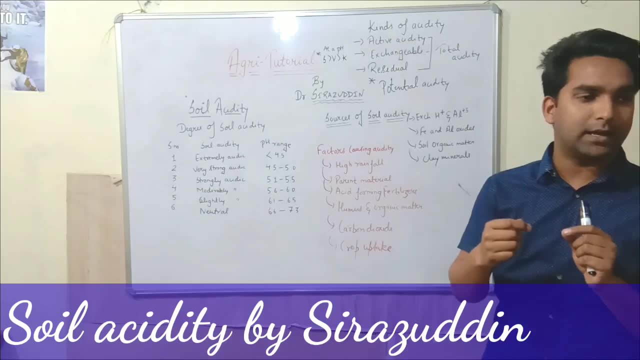 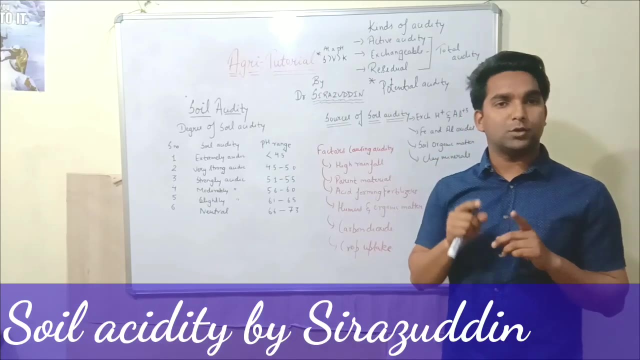 so whatever hydrogen or aluminium ions are present in your soil solution, you know, mind it. whatever soil is present in the solution due to them, the acidity that is termed as acidity is active acidity. so generally when you do analysis in your lab of your soil, so basically the pH that your pH meter measures. 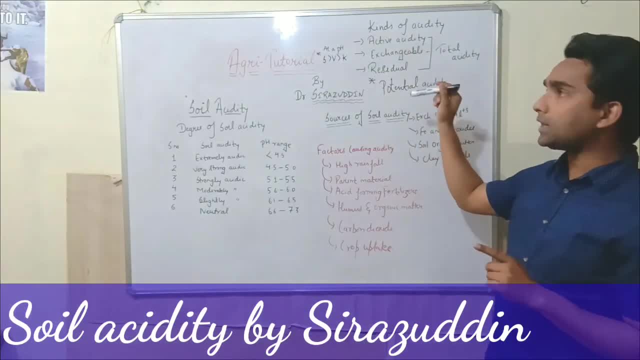 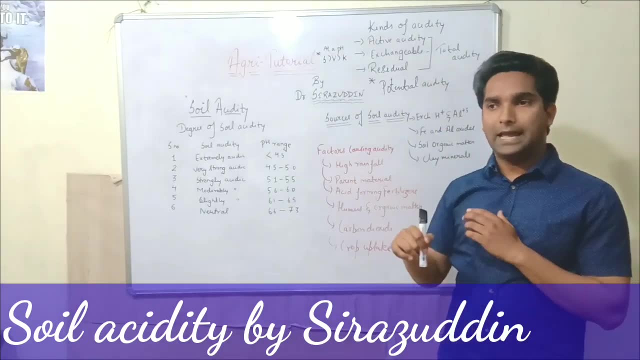 that is only active acidity. we never, you know, take care of the exchangeable and the residual activity while we go for the analysis of pH in the lab. so active acidity is read out by your pH meter. ok, why? because it reads out the hydrogen and aluminium ion concentration. 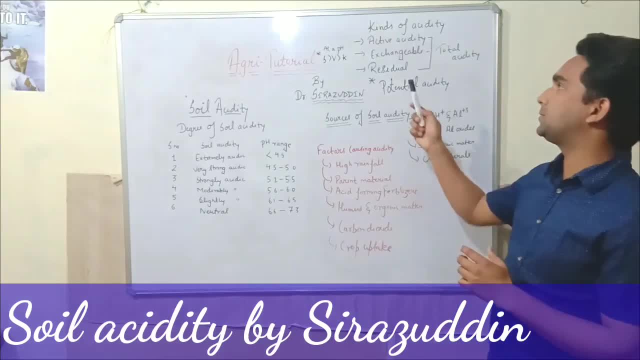 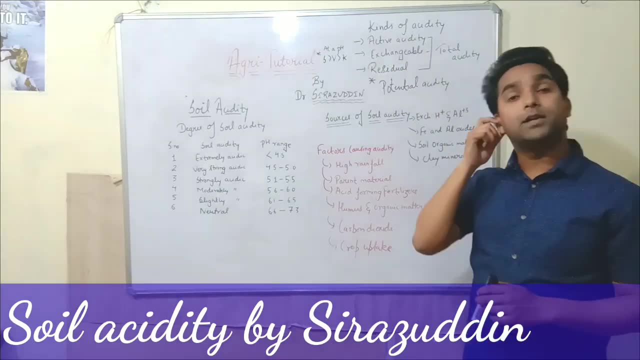 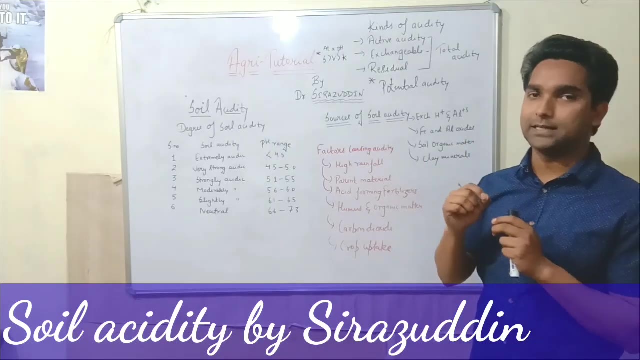 of the soil solution and that will be displaced at the pH meter as an active acidity. now this exchangeable acidity. it is also known as salt replaceable acidity, mind it. so what is the synonym of this salt replaceable acidity? so now we are getting to know. 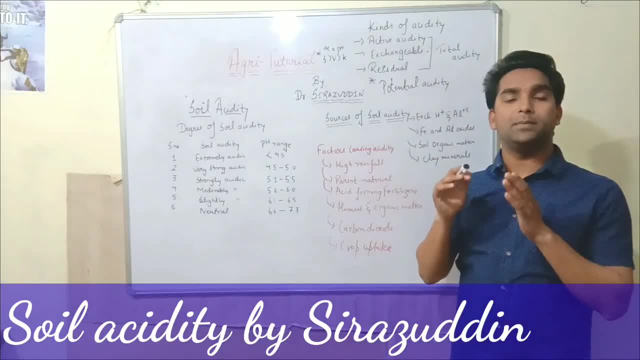 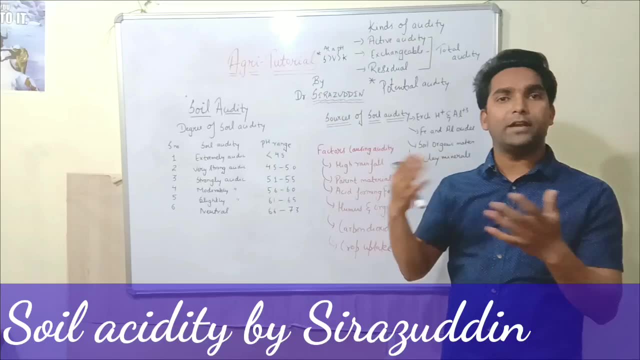 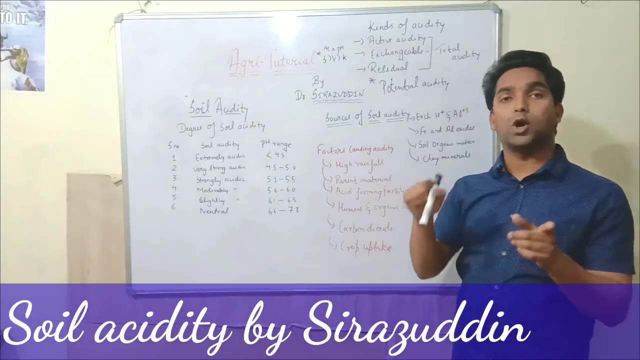 exchangeable acidity, that all the hydrogen and aluminium ions which are present in your soil colloids- and they are, you know they are free to exchange. so the acidity that will come from them that will be termed as exchangeable acidity. so all the hydrogen and aluminium ions. 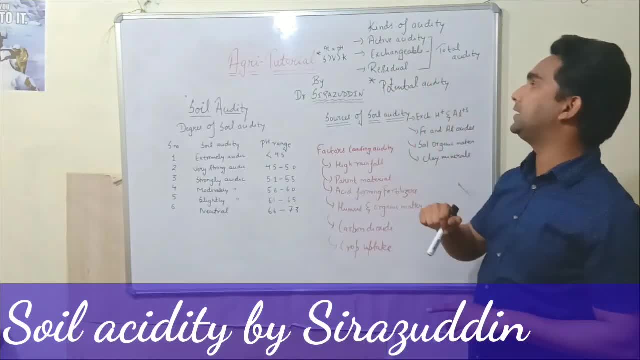 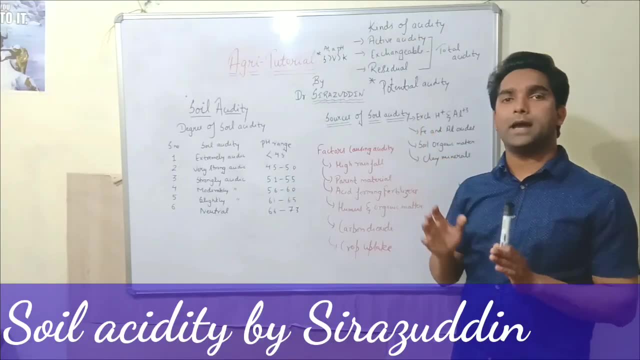 on your soil, colloids. that will be termed as exchangeable acidity. then, moving on, the third one is residual acidity. so we can call this all your hydrogen ions, all your aluminium ions, even your aluminium oxides or hydro oxides, which are present in your non exchangeable forms. 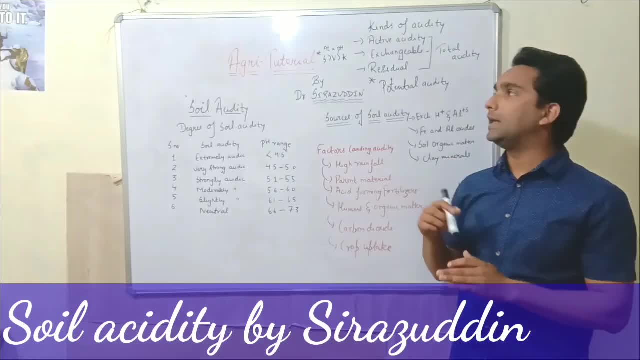 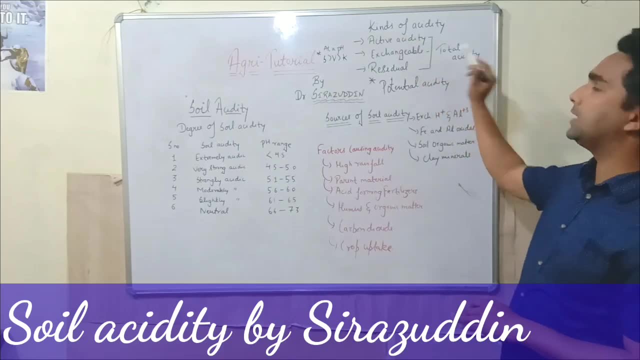 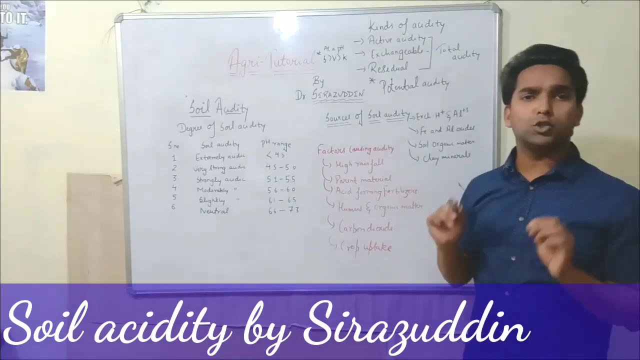 in clay or on organic matter. that is termed as the residual acidity and the sum of these three is termed as total acidity. now one more question is asked. that your active acidity, basically its pool, is very narrow and very small. but it is small, but it is the most important. 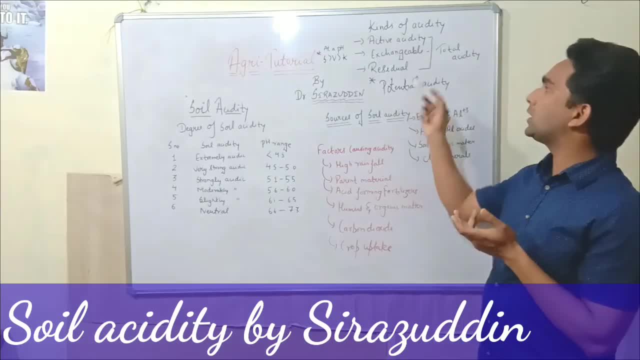 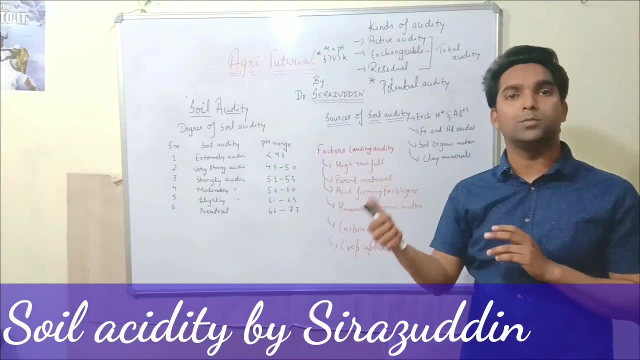 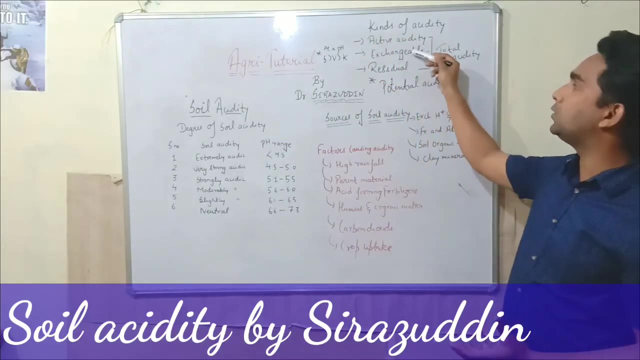 in terms of agriculture. why? because your active acidity that only decides the soil solution environment, for the plants and for the microbes as well. so to say, its potential or its pool is very small as compared to exchangeable and residual, and the pool of exchangeable is very high. 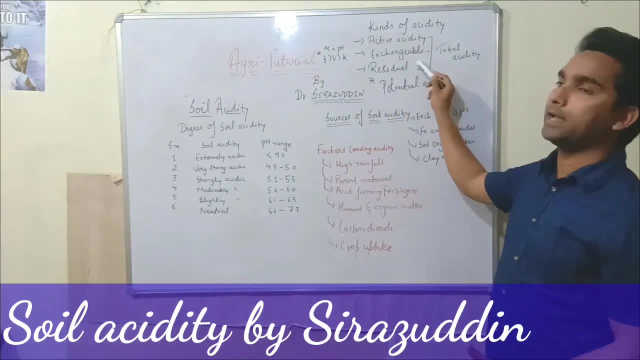 as compared to active, but the most important is considered as residual, so the pool of residual acidity will be the highest. okay, then you might have seen that I have put one more star out. that is potential acidity. so this is a very less common form of the acidity. 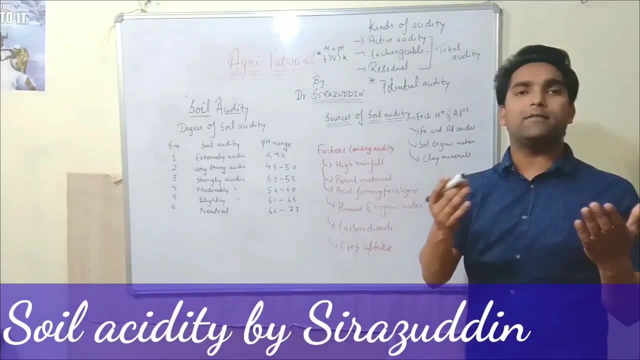 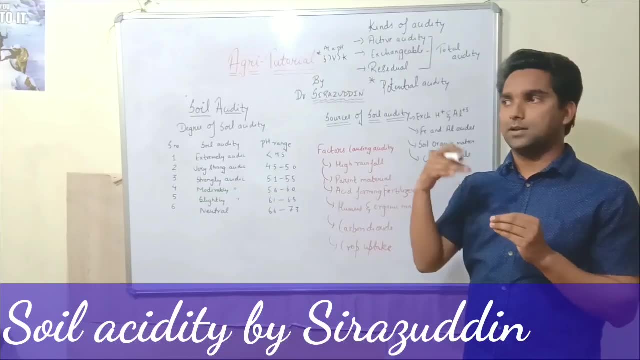 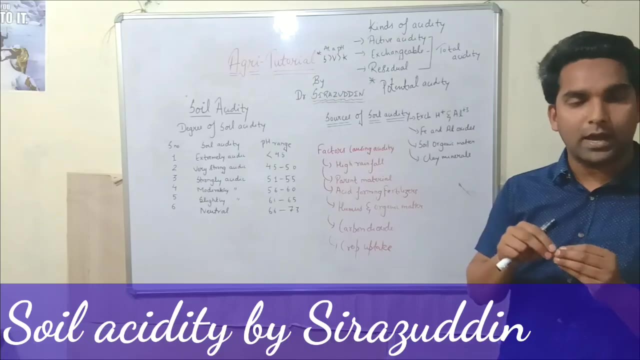 but what is potential acidity? you may have heard the term cat craze or acid sulphate soils. so if ever your sulphur compounds get oxidation, that also causes acidity. so whenever sulphur compounds get oxidation and because of that the acidity that is termed as potential acidity. 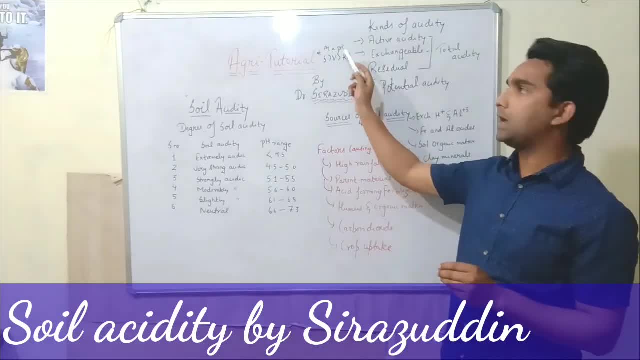 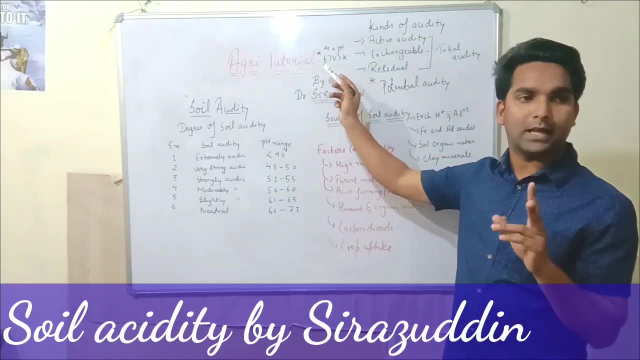 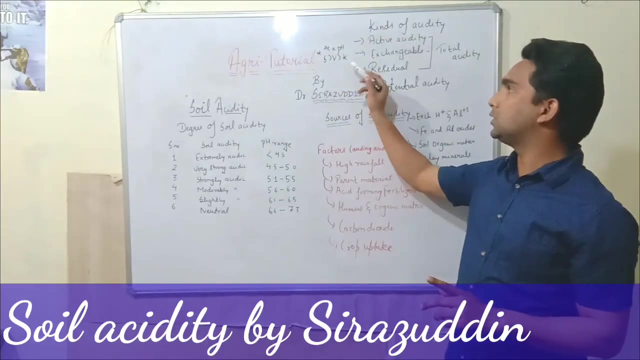 now you will see here, at a particular pH, if we talk about exchangeable acidity. so in the smectite group the most exchangeable acidity will be found, followed by vermiculite, and the last one is your kaolinite. so this has to be, you know, like. 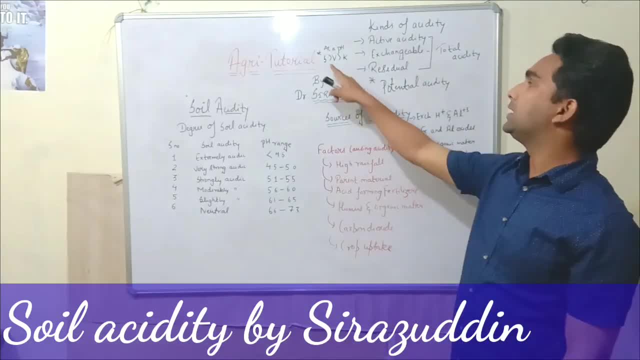 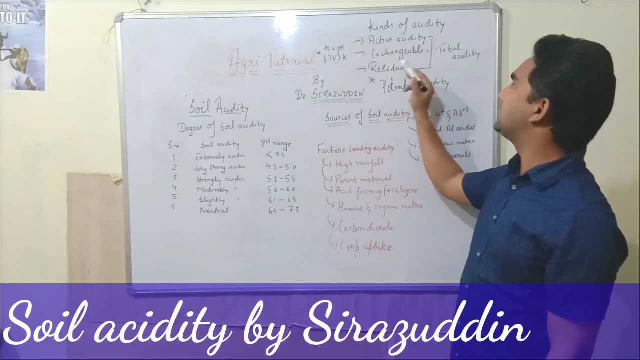 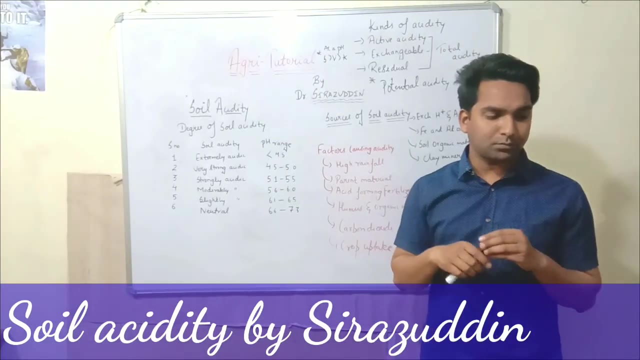 this has to be remembered by you- that smectite, followed by vermiculite and then kaolinite at a particular pH, the exchangeable acidity follows, like this: okay then, moreover, one more point is asked. a lot we know that the residual acidity- this is commonly